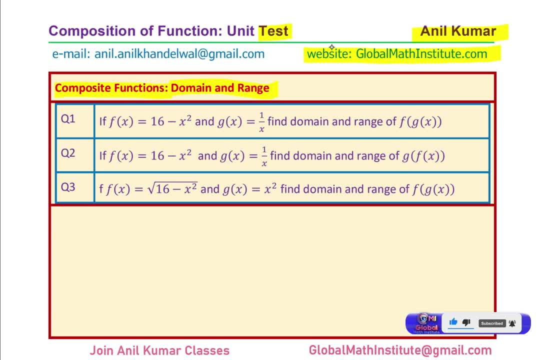 So let us see how do we answer these questions. I will actually use two different strategies to do the first one, which is very simple, just to get these strategies right. So let us say we have a domain and range of f, of g of x and then of g of f of x. 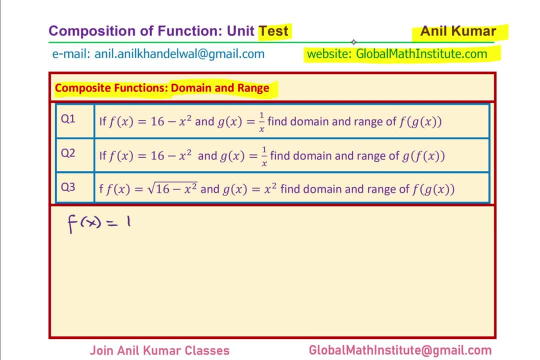 So we are given f of x is equal to 16 minus x squared. Well, that is question number one we are trying to do now. And we are given g of x is equal to 1 over x. We need to find domain and range of f of g of x. 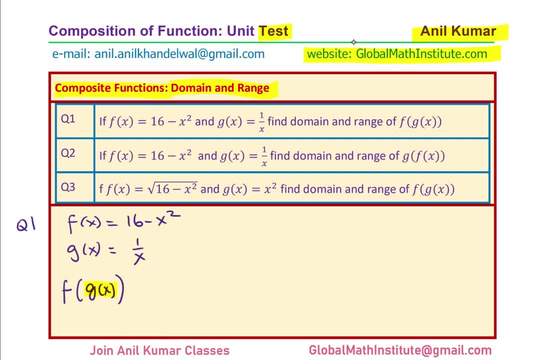 Always look into the inside function first. So g of x is given to you as 1 over x. So of course there is one restriction there, and that is that x is not equal to 0. Perfect, So we do get restriction for the composite function. 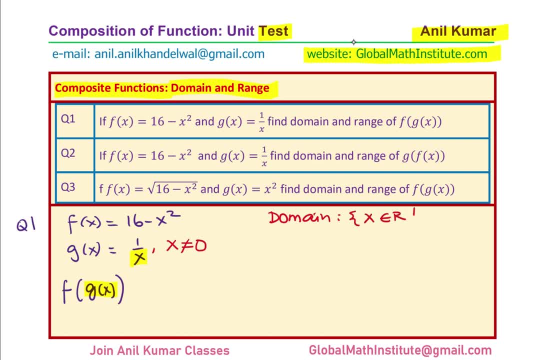 And therefore the domain can be now written as: x belongs to real numbers where x is not equal to 0.. Is that clear, Perfect, right? You will also notice that for 1 over x, output cannot be 0, right. 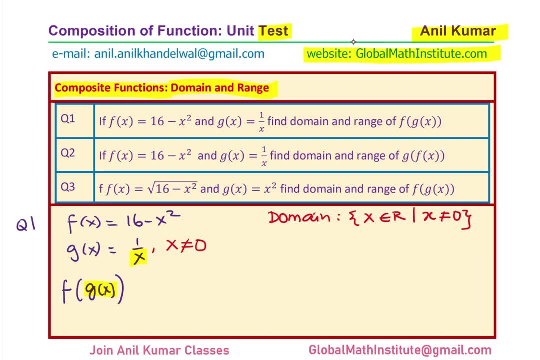 Can you tell me how that is going to affect the range of this particular composite function? Well, f of g of x is 16 minus x squared, And if the input does not have 0, then the value of 16 is not possible, right. 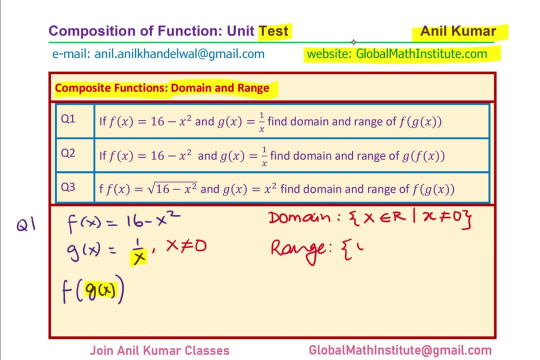 And therefore the range should be less than 16.. Make sense. So range will be: y belongs to real numbers where y is less than 16.. Correct. Now here is alternate way of doing the same question. You could actually write down the combination. 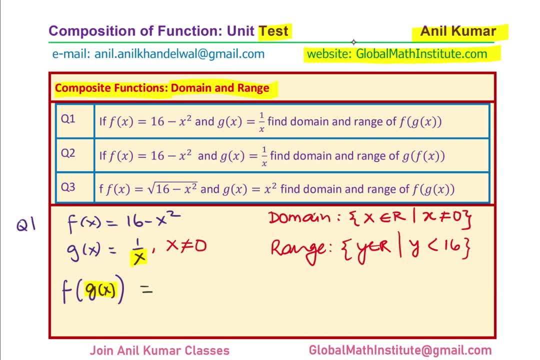 You could actually write down the composite function f of g of x, Replacing x with 1 over x. you get what You get: 16 minus 1 over x squared, correct? What do you notice? Well, 1 over x squared is always positive, so the maximum value can be 16.. 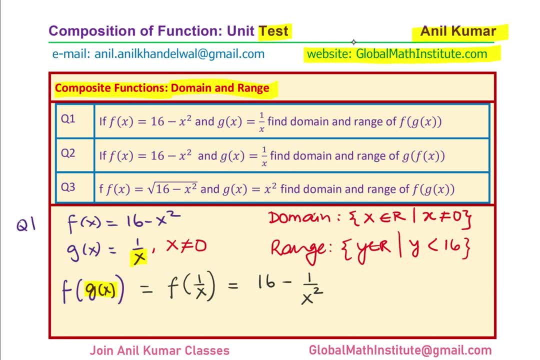 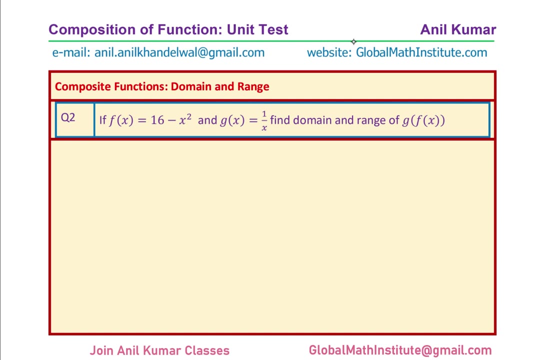 But 1 over x squared cannot be 0, so the maximum value of 16 is not possible And therefore all the values below 16 are possible. so that becomes our range Make sense. So that is how we can find domain range of this particular function. 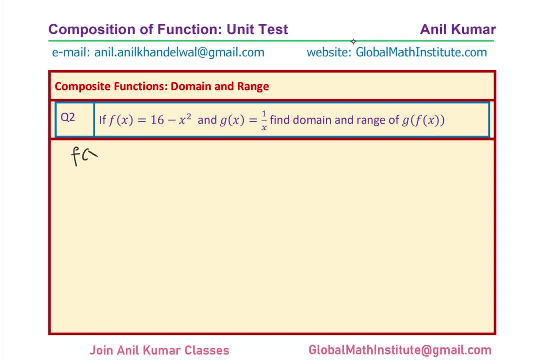 Now let us move on and answer question number 2.. So I hope the concepts are absolutely clear, right? Once again, let us write down the functions: f of x is 16 minus x. squared g of x is 1 over x. 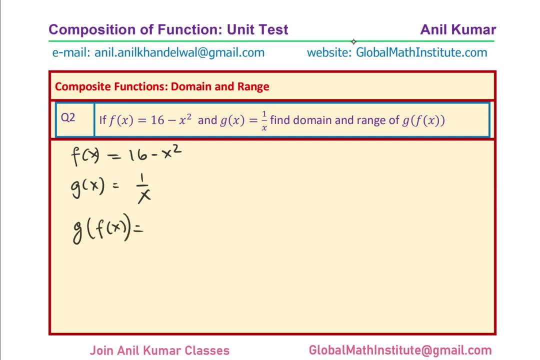 And what is f of g of x? It is going to be 1 over 16 minus x squared right. So g of f of x is 1 over 16 minus x squared. It is a good idea to write down the function f of x. 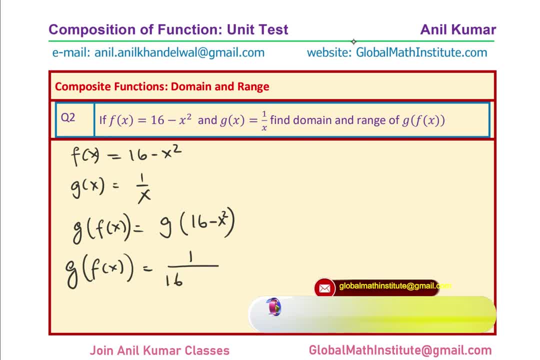 So g of f of x is 1 over 16 minus x squared. It is a good idea to sketch this function and then look into domain range. Well, that could be a very important strategy. Denometer cannot be 0. That means x cannot be equal to plus and minus 4.. 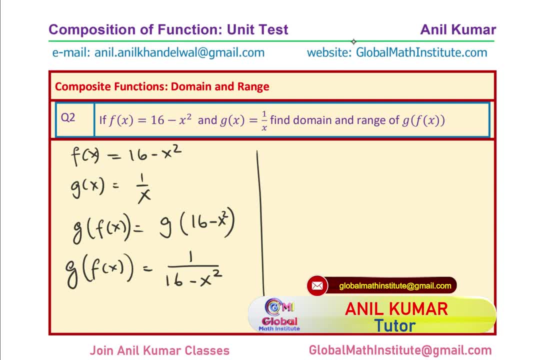 And that gives us our domain right. Clear, So clearly. the domain is that x can have all the real numbers except plus and minus 4.. So that becomes the domain right. So if you sketch this function, what do you notice? 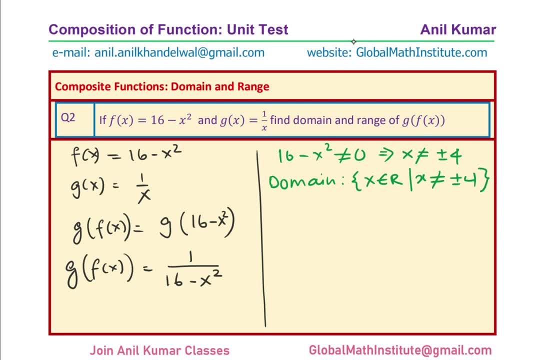 At plus and minus 4, you get vertical asymptotes right To sketch 1 over 16 minus x squared. I will appreciate if you could pause the video and first sketch 16 minus x squared and then its reciprocal. I hope you got the graph. 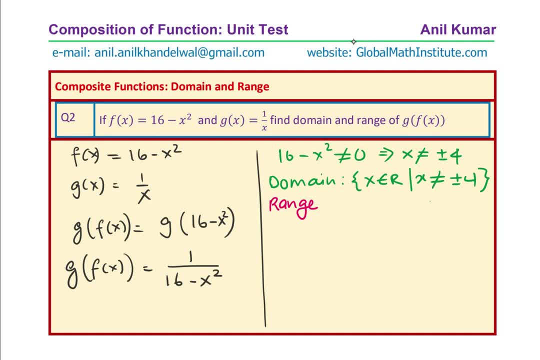 And now you can write down the range of this graph. Write down the range of this composite function. Perfect. So the parabola opening downwards with maximum value of 16, here is the graph to see how do we find the range of this particular function. 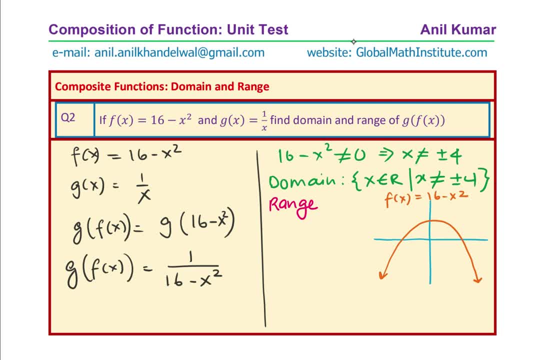 The minimum value at the center will be 1 over 16, right, And on the other side we have the function as shown, which is approaching 0 from the negative side. So we can write down the range of this particular function. 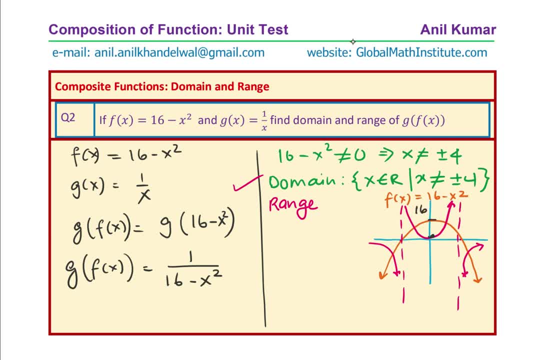 So we can write down the range of this particular function. So y is always greater than or equal to 1 over 16, or it is less than 0, right? So that's how you get domain and range of this composite function. 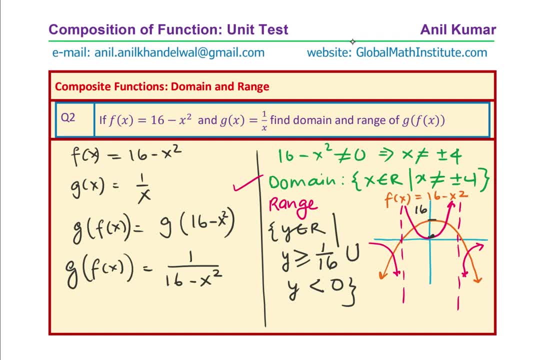 Clearly the solutions of question number 1 and 2, they are very, very different, right? So now let us take up the solution for question number 3.. So now let us take up the solution for question number 3.. 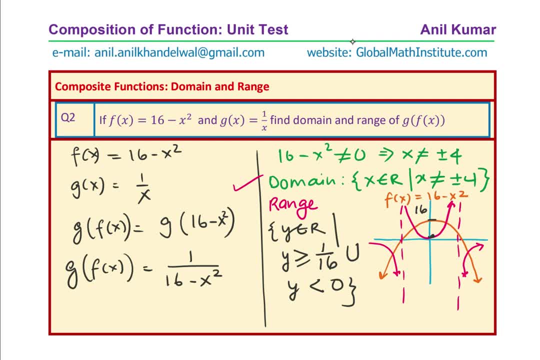 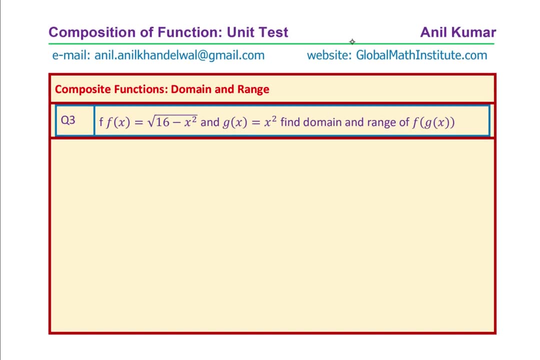 So now let us take up the solution for question number 3.. You can write down the composite function and then the domain and range of this particular question. We are given f of x as equal to square root of 16 minus x squared. 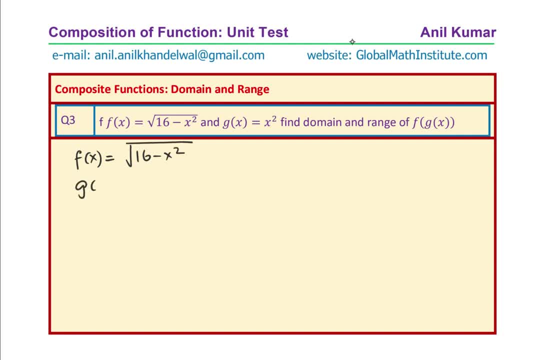 g of x is equal to x squared and the function is f of g of x, the composite function which clearly is square root of 16 minus x to the power of 4, x squared squared, correct. Now can you write down domain and range? 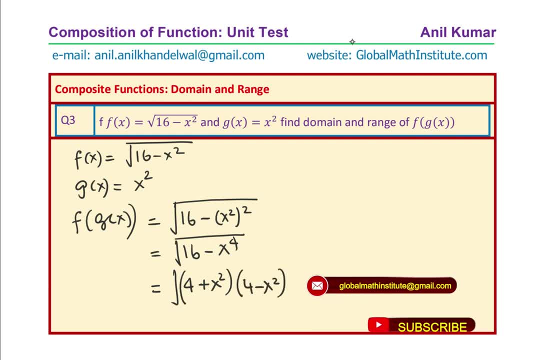 We are factoring to show you that 4 plus x squared and 4 minus x squared are the two factors. a squared minus b squared is a plus b times 4, a squared minus b squared is a plus b times a minus b. 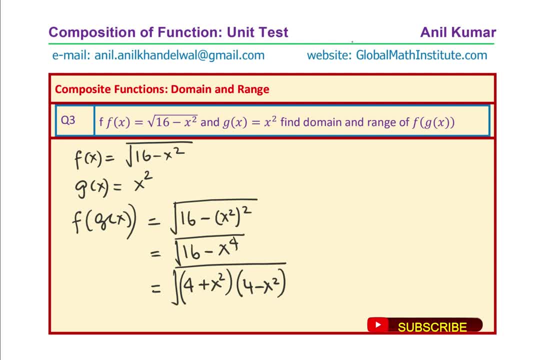 the first factor is always positive. the second factor could be negative: 4 minus x squared. We have to maintain it to be positive. So that is to say that 4 minus x squared should be always greater than equal to 0. And that really means that. 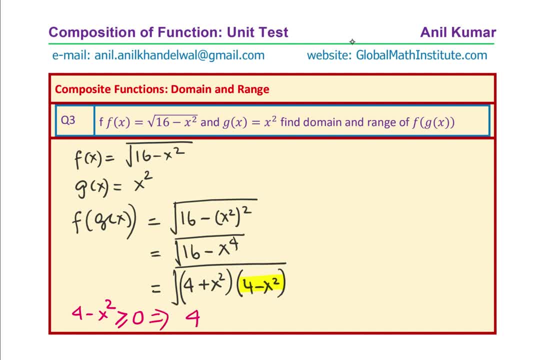 is greater than equal to x square right, or X is between plus and minus 2, so now we are in a position to write down the domain. you can pause the video, write down domain and range and then check with my answer. as expected, the domain is all real numbers where X is between plus and. 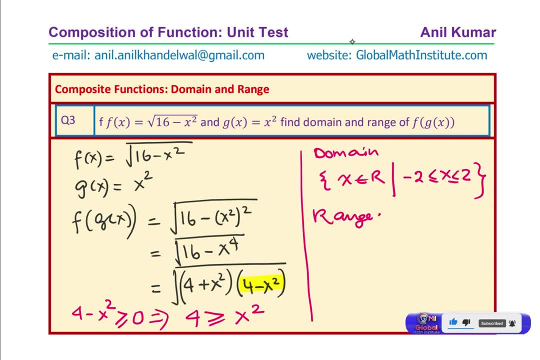 minus 2. how about the range? well, the maximum value could be square root of 16, right, and the minimum, of course, will be 0, square root of 16 being 4. so Y is less than equal to 4, but greater than equal to 0.